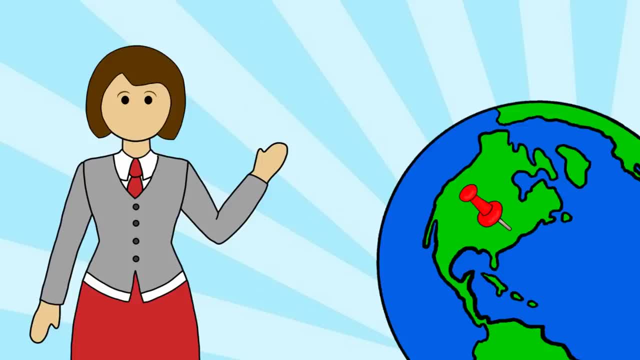 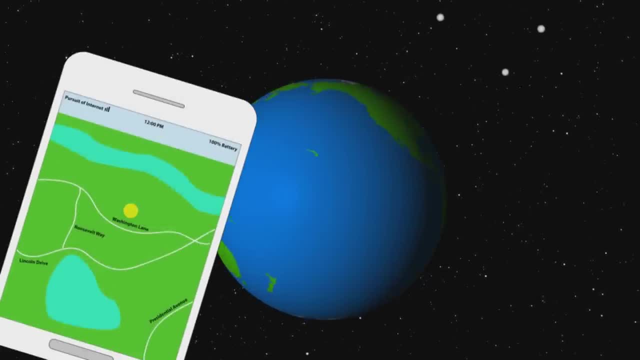 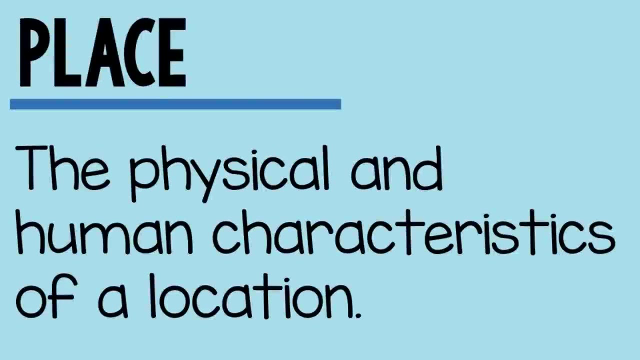 Lines of latitude and longitude meet at specific points, called coordinates. By typing in specific coordinates on your cell phone, you can find an exact point on the planet, no matter where you are. Place describes the characteristics of a location. Are there mountains, beaches, valleys or deserts? 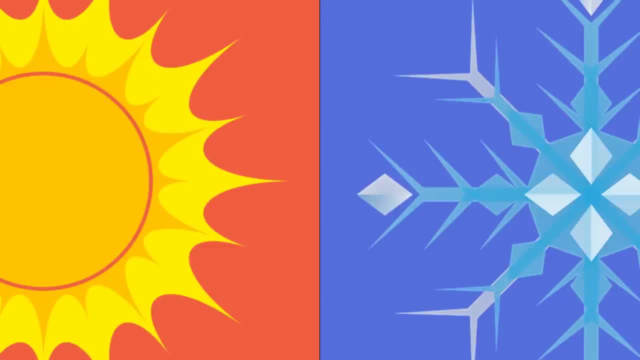 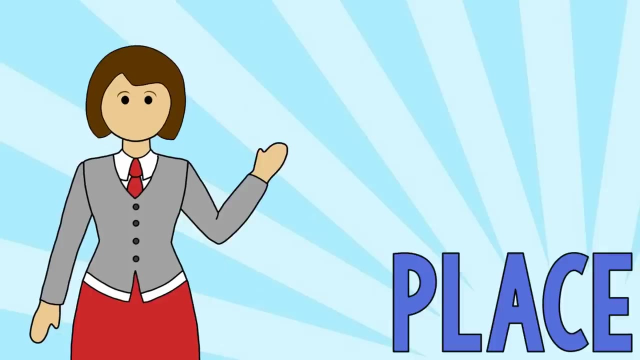 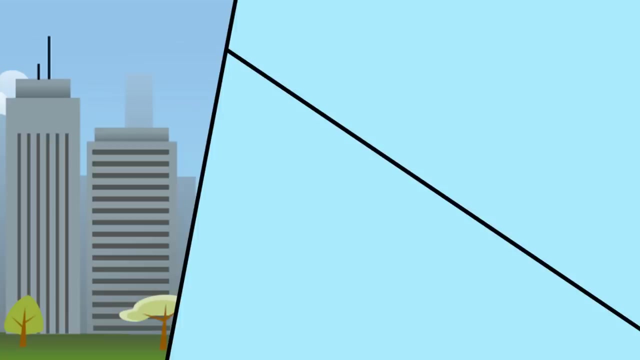 What is the climate like? Is it hot or cold? Do you see forests, sand, grass? The theme of place doesn't only describe physical characteristics, but human characteristics too. How are people using the location? Do you see major cities? What do the houses look like? 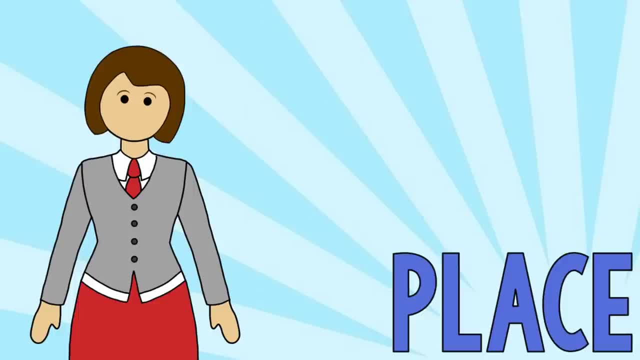 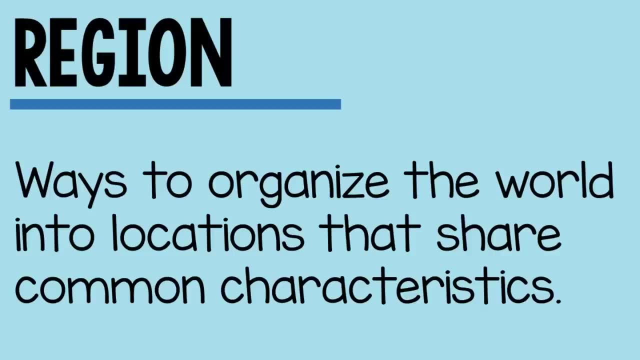 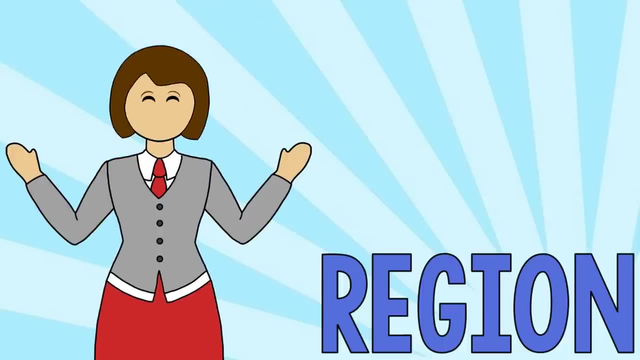 Is there lots of farmland or densely populated neighborhoods? How is the geography affecting the way people live their lives? Regions are ways to organize the world into locations that share common characteristics. You can organize places many different ways, from time zones to geographic characteristics, economic similarities, languages spoken. 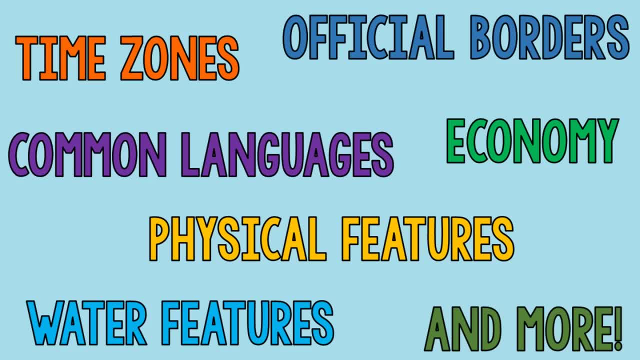 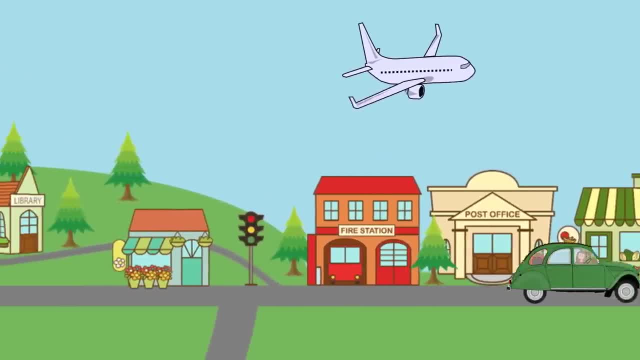 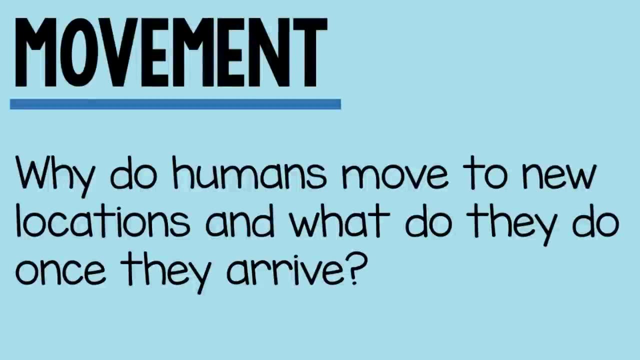 the official borders of countries, cities, towns and much, much more. Humans are always on the move and they're taking ideas and goods with them. When studying movement and geography, ask yourself: Why did people move to that area? How did they get there? 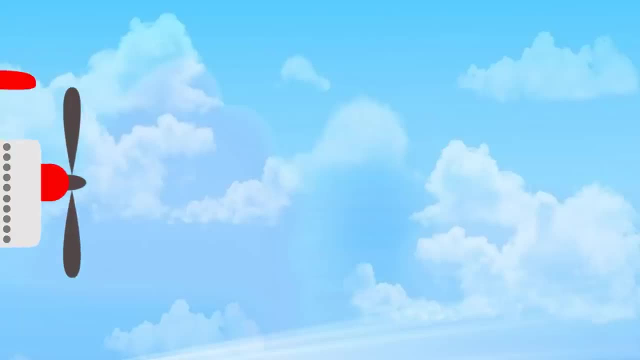 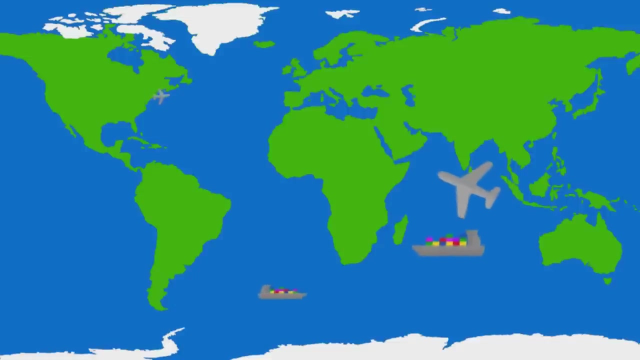 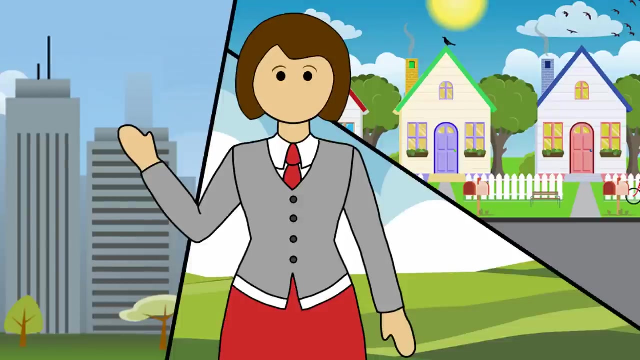 What items or ideas do they take with them? What did people do once they moved to a new location? Movement doesn't just apply to people either. It applies to goods, ideas and information being transferred from place to place too. How does the new information or ideas impact a location after it's transferred? 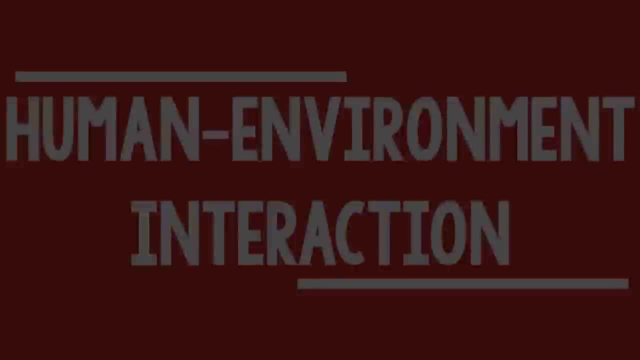 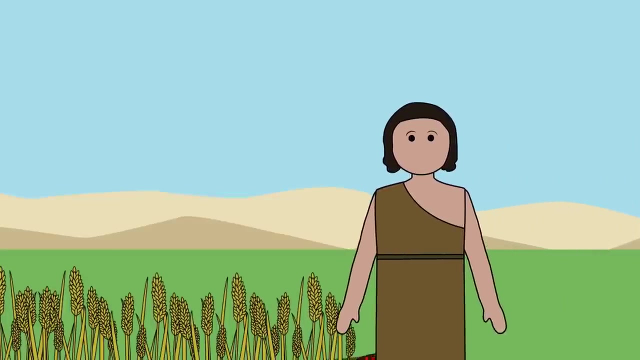 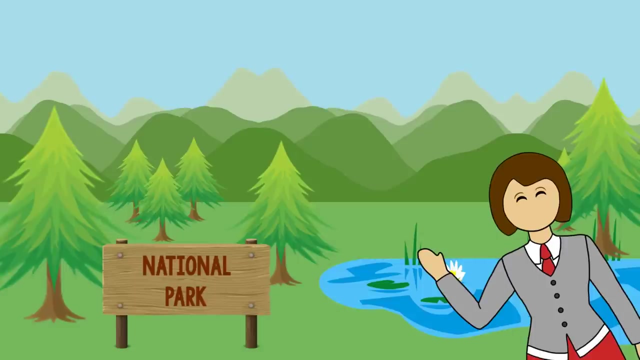 So many questions. It's undeniable that humans impact the environment wherever they go. Since the dawn of time, humans have changed the environment to fit their needs. They've built homes, towns and cities. They've protected lands for future generations and used others to plant crops or build businesses. 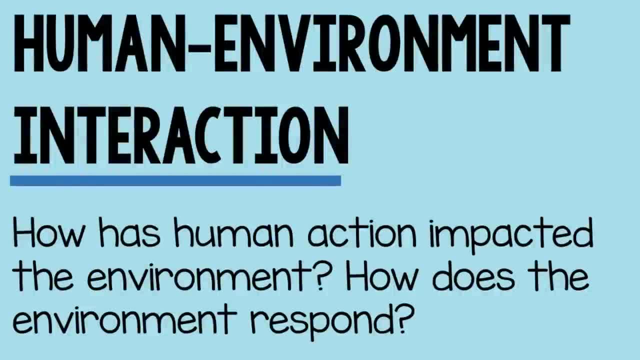 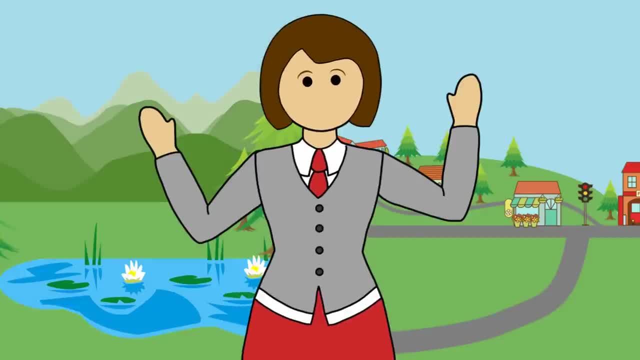 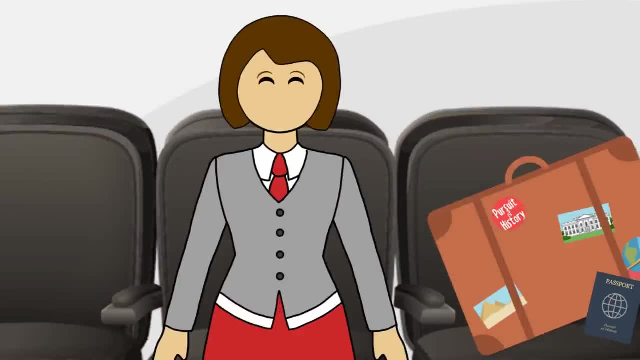 How has human action impacted the environment? How does the environment respond to these changes? The relationship between humans and the environment is constantly changing, as one reacts to the other. Oh, looks like we've landed. Who knew the five themes of geography could be so fascinating?